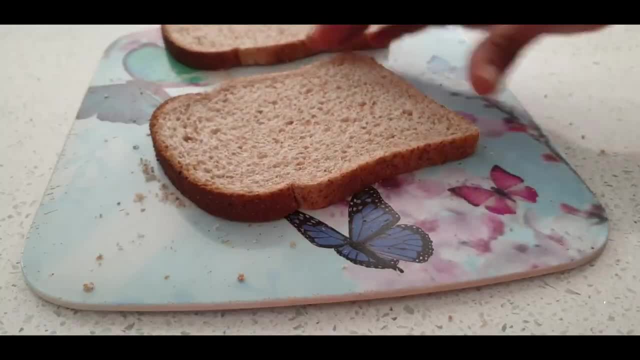 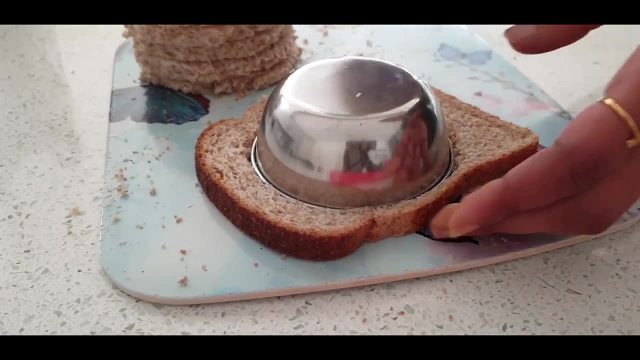 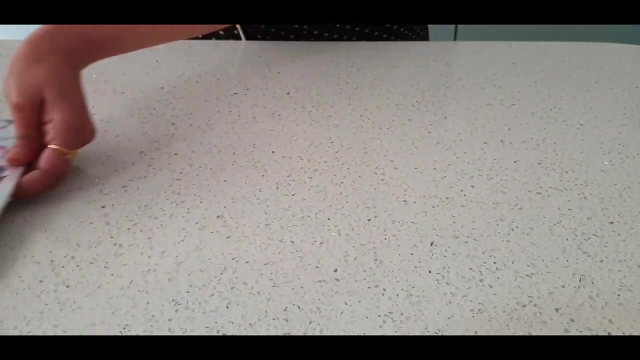 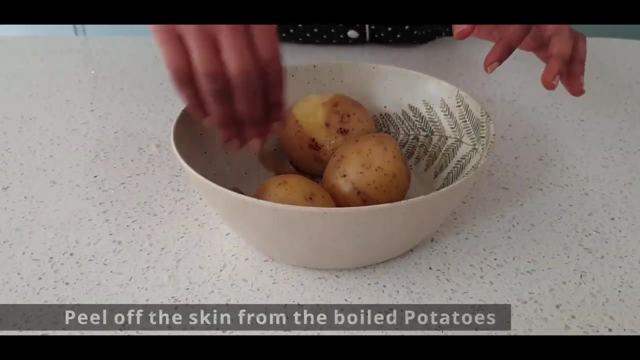 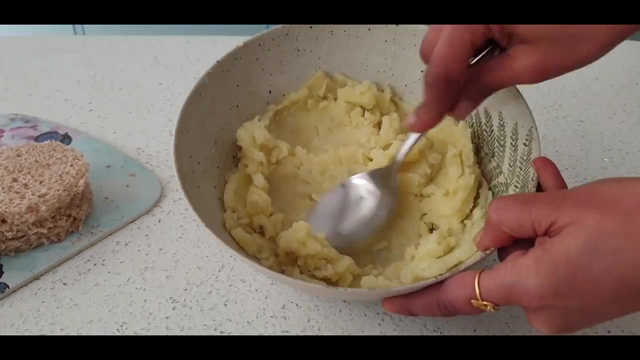 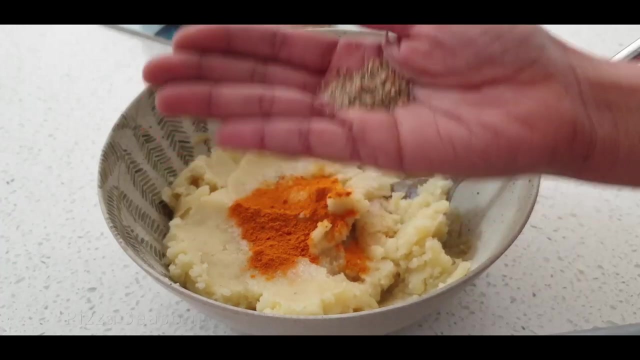 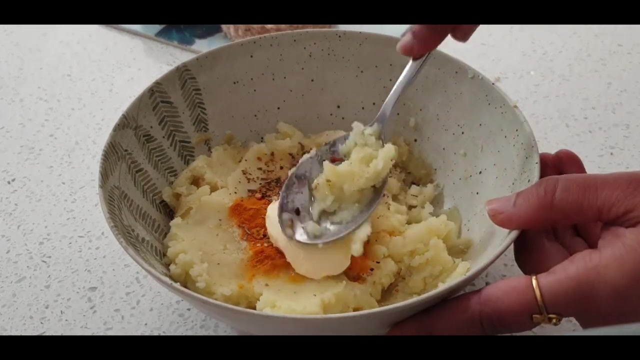 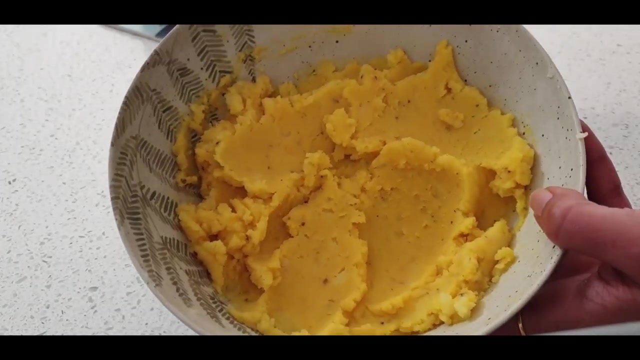 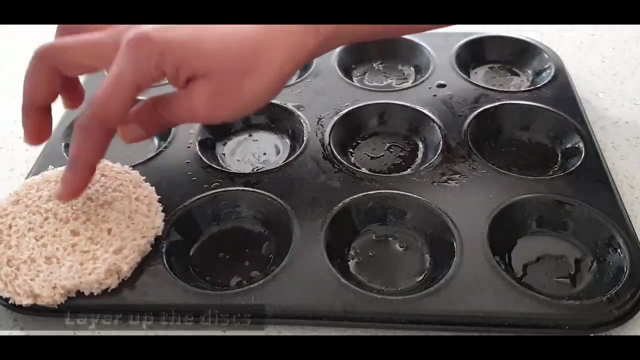 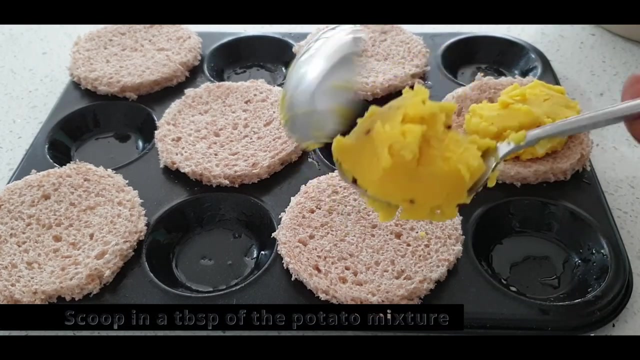 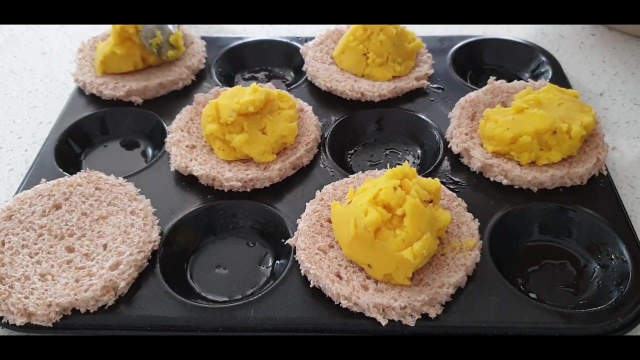 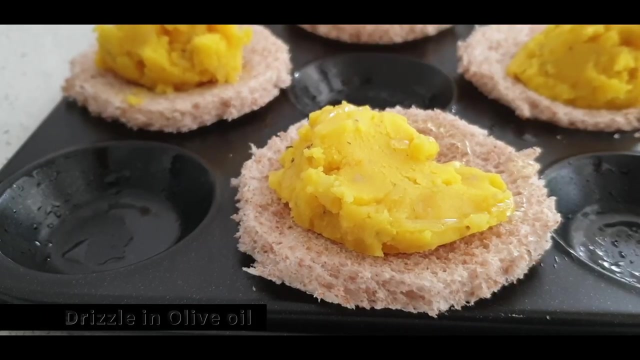 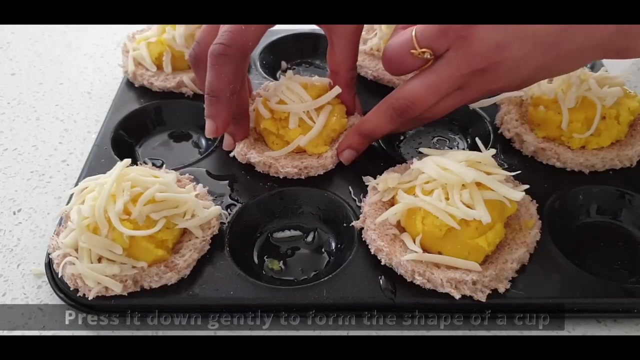 Thank you so much for watching. I'll see you in the next video, Bye, bye. Thank you for watching. I'll see you in the next video. Bye, bye. I'll see you in the next video. Bye, bye. Thank you for watching. I'll see you in the next video. Bye, bye. 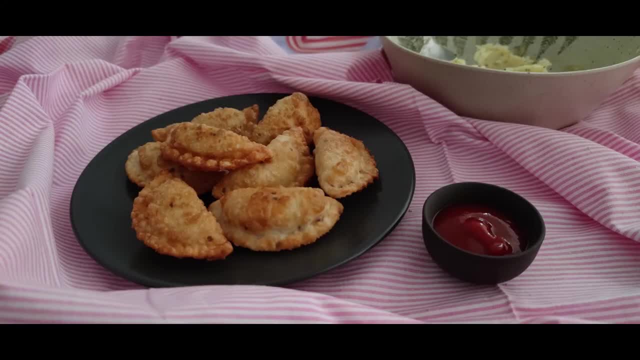 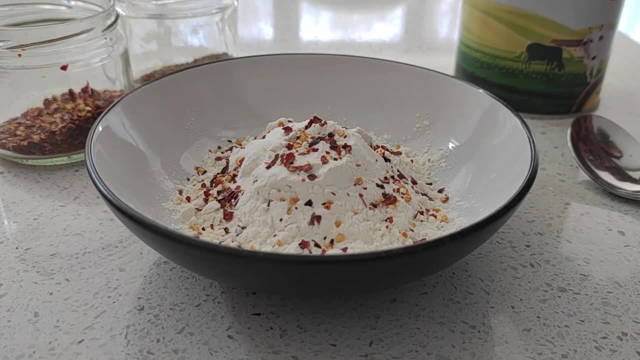 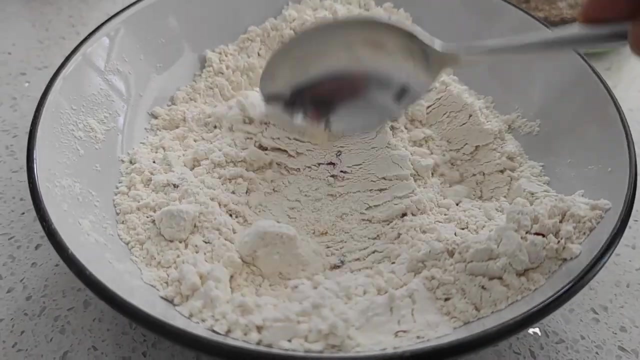 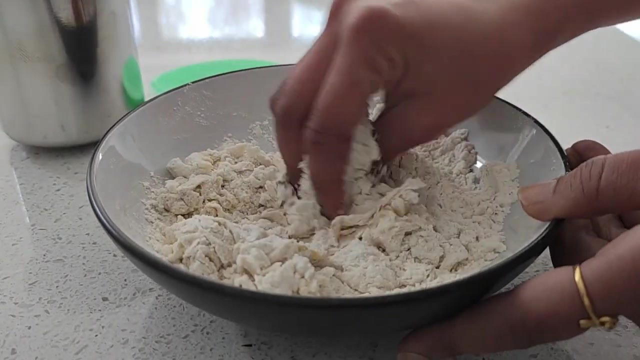 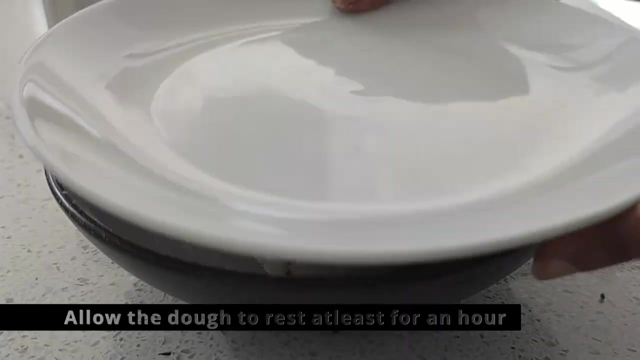 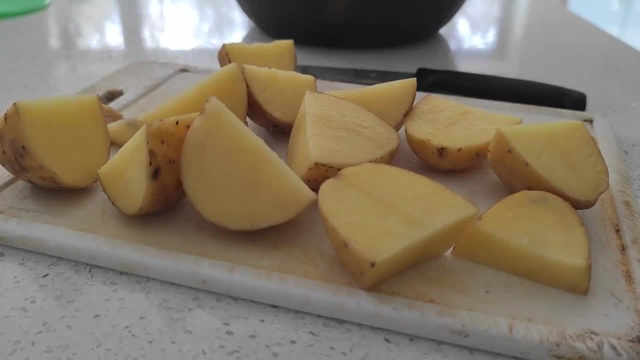 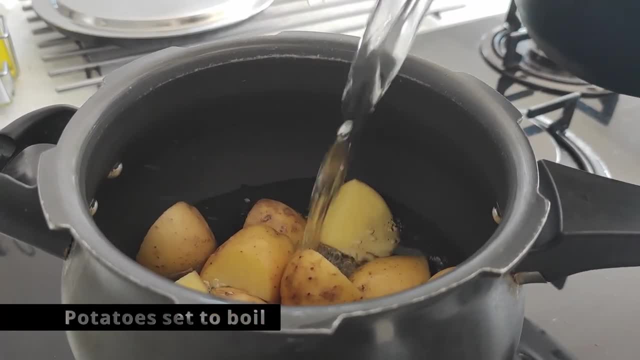 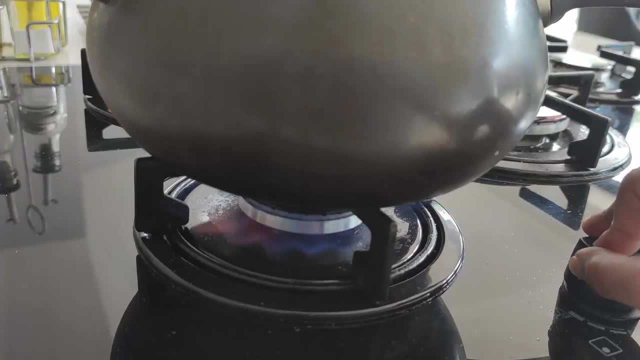 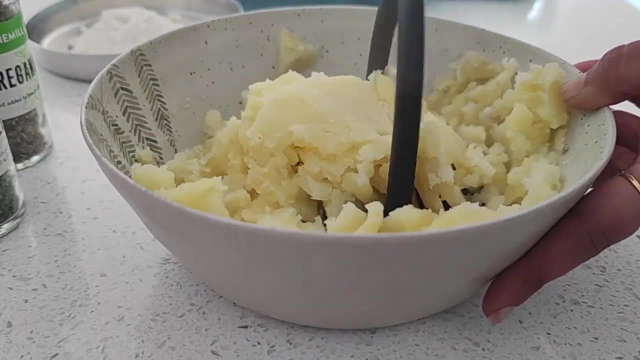 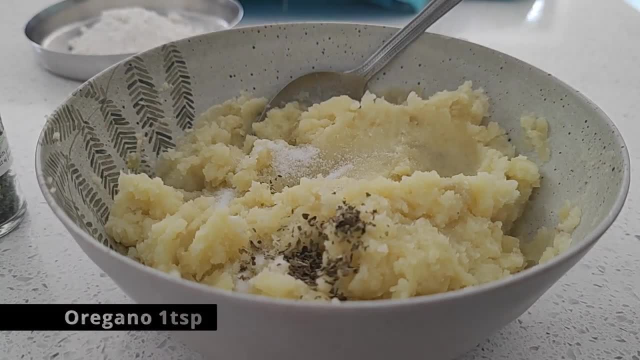 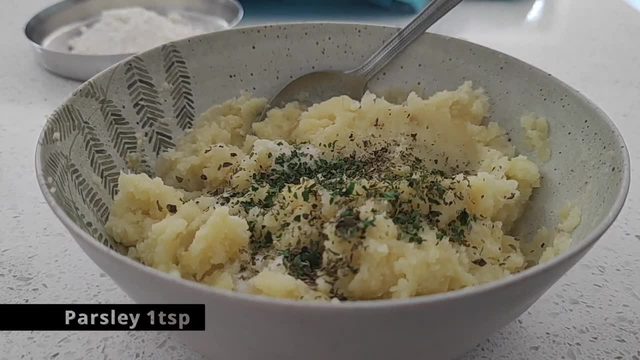 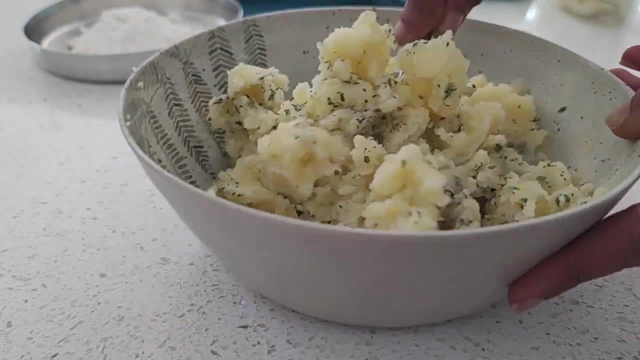 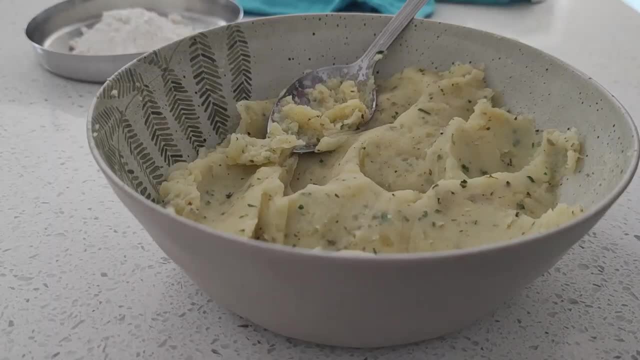 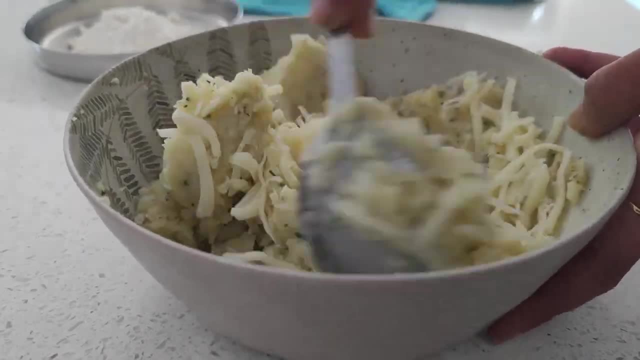 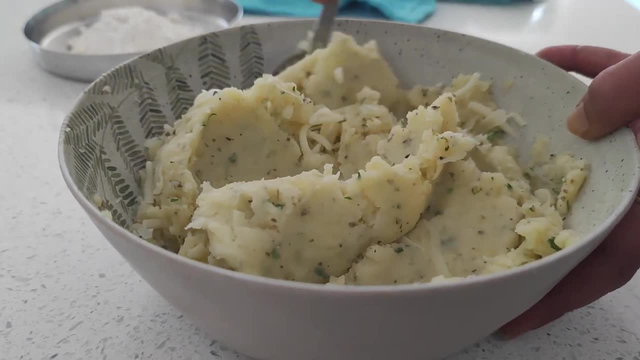 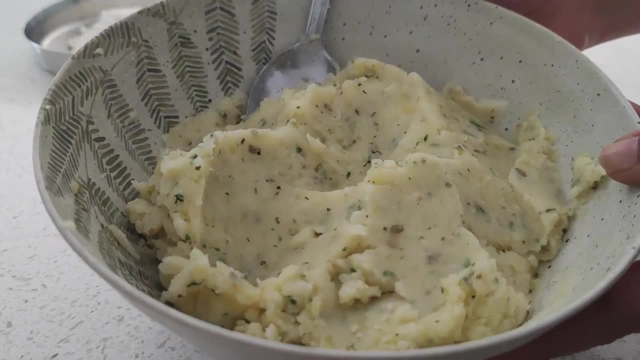 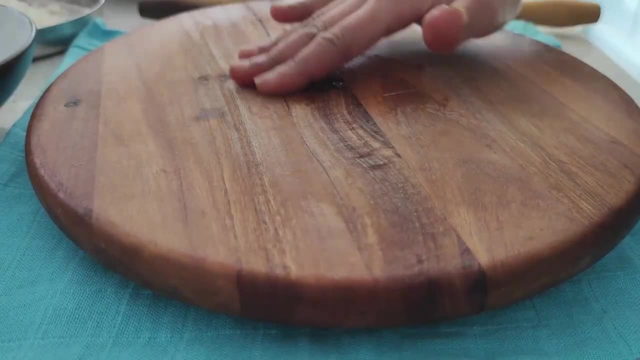 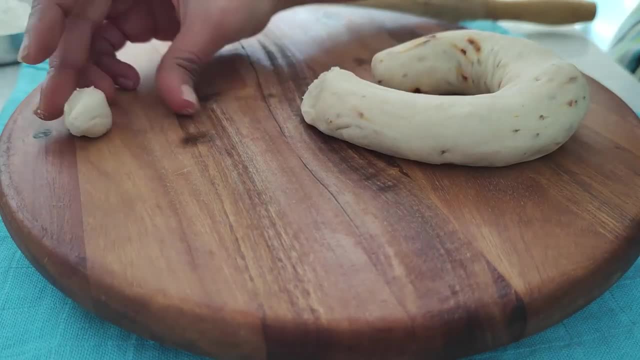 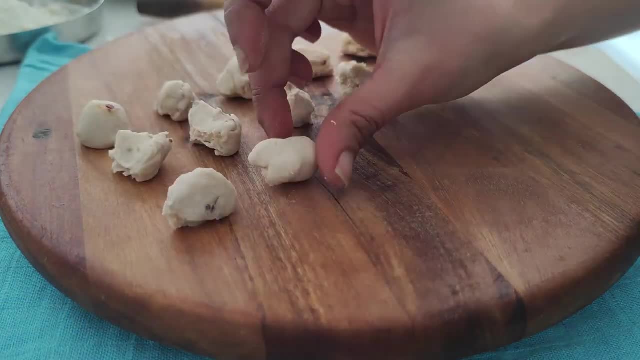 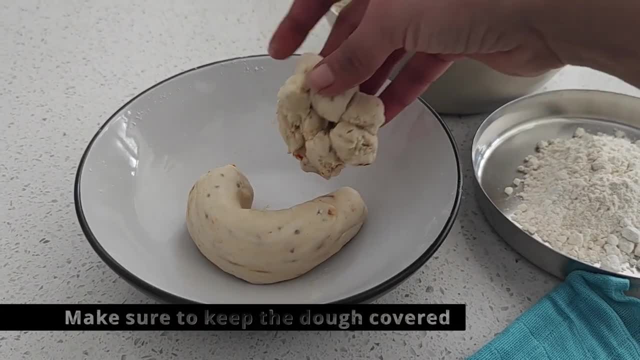 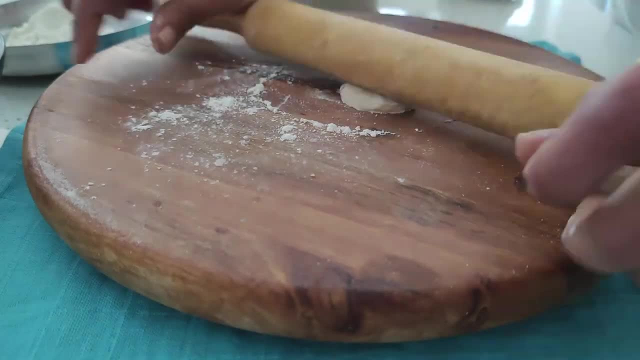 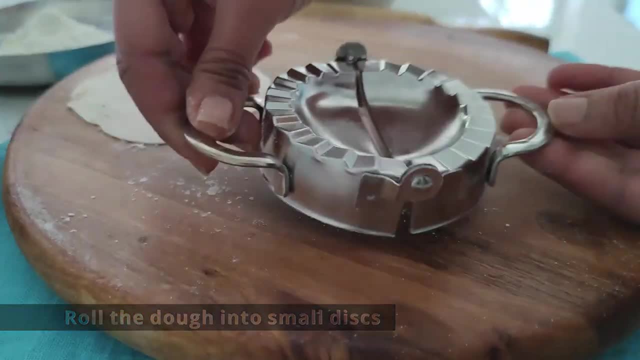 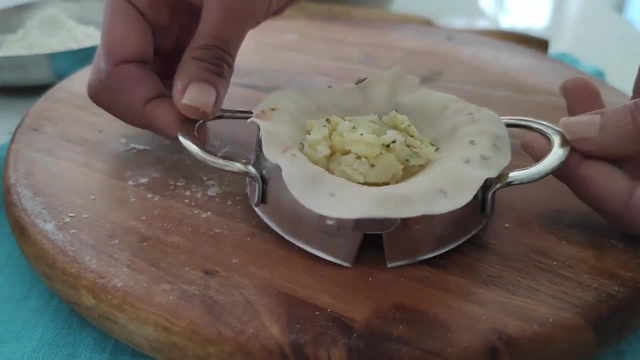 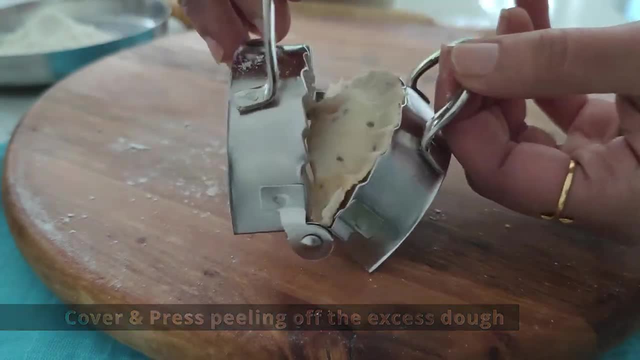 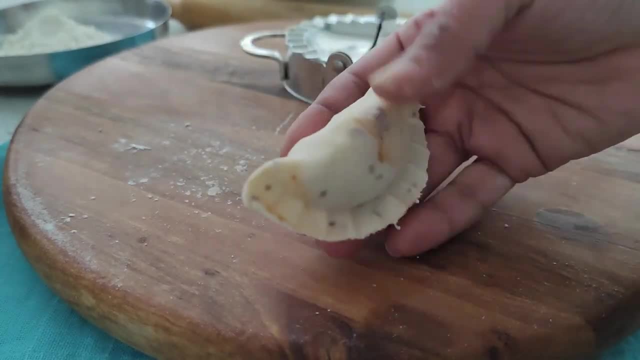 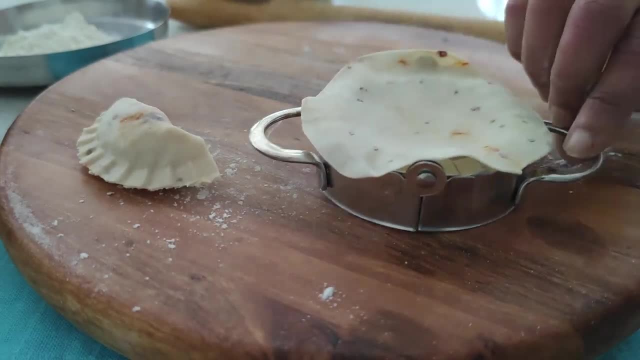 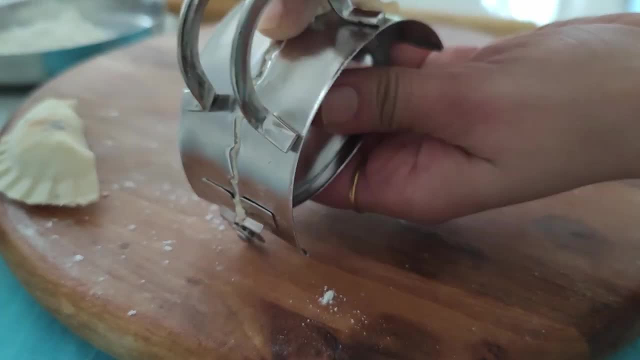 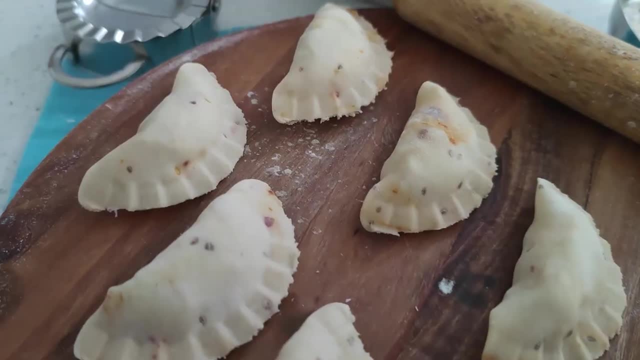 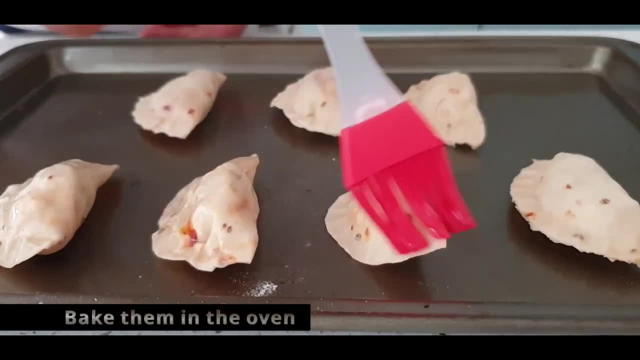 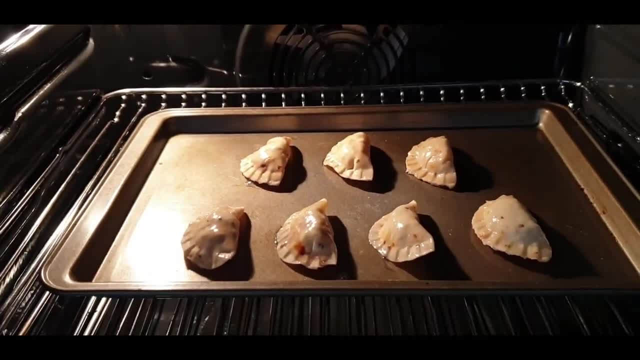 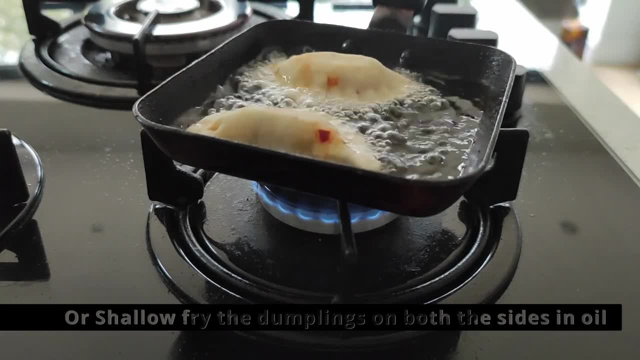 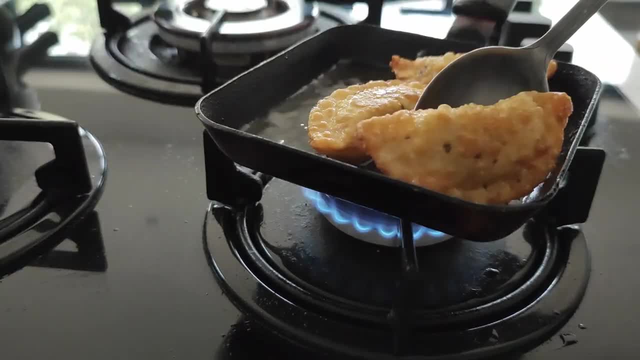 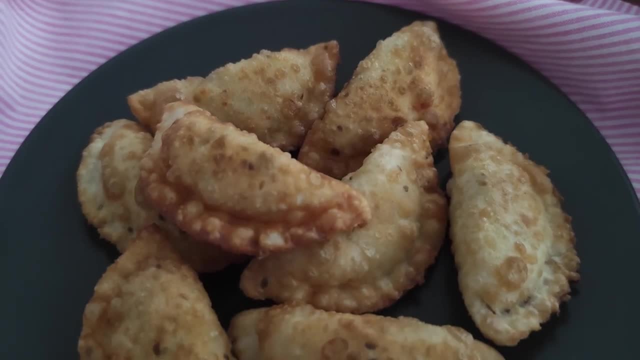 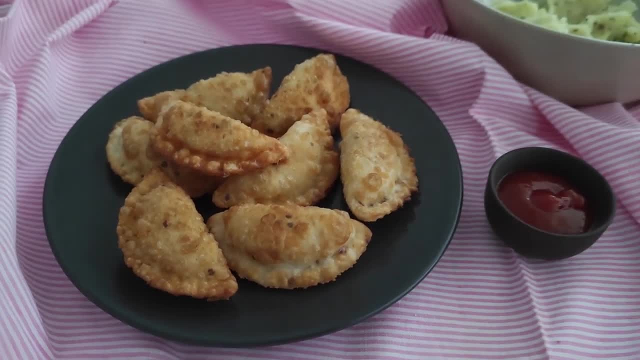 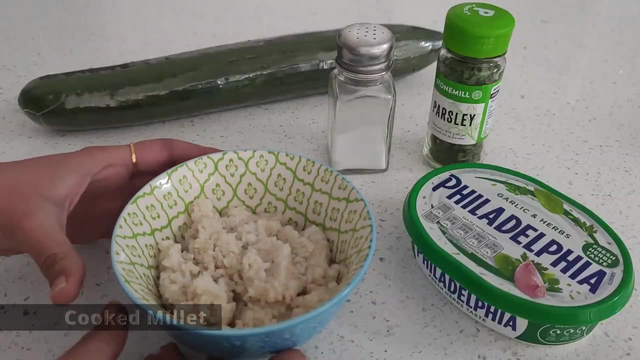 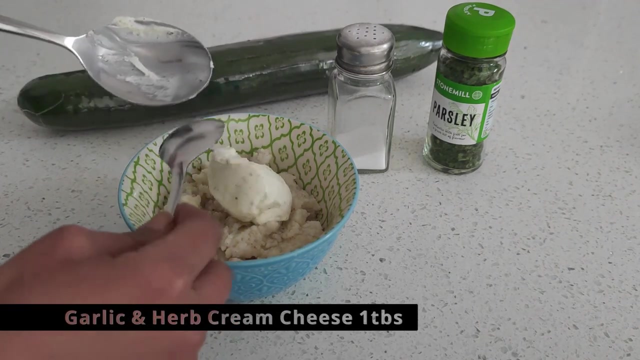 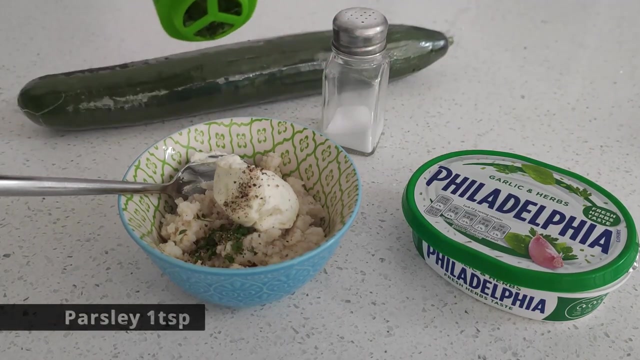 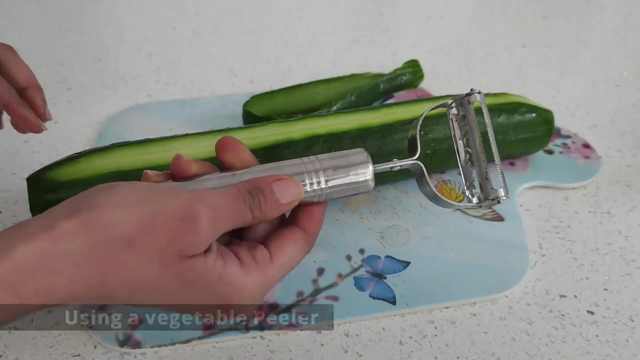 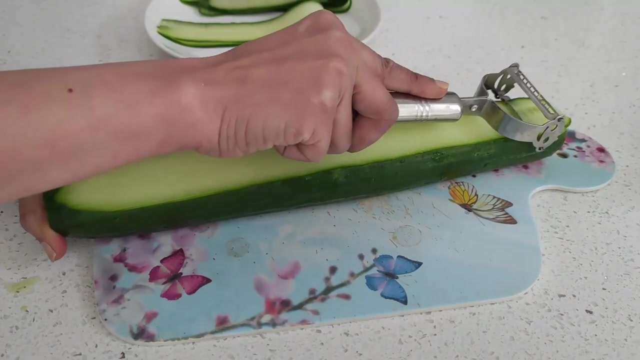 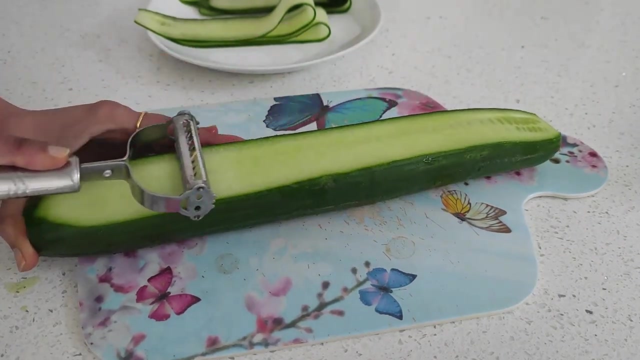 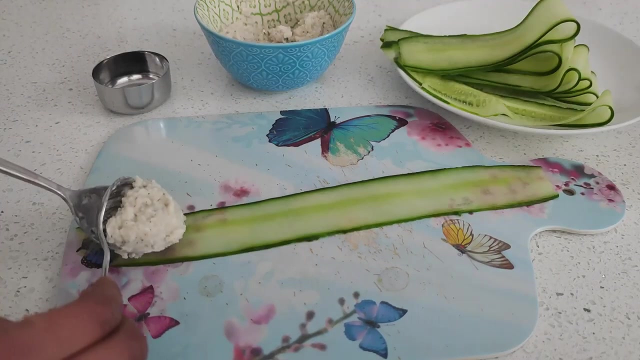 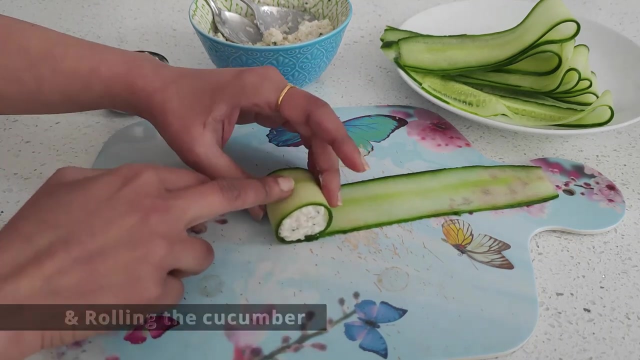 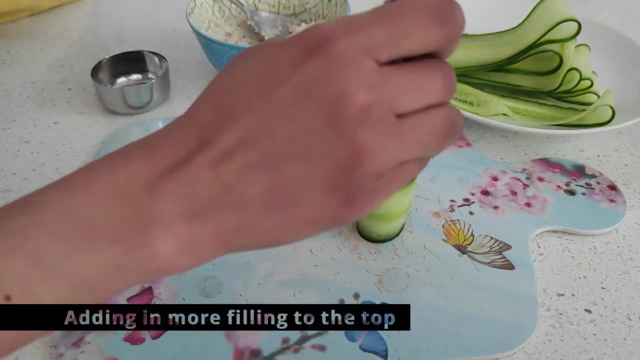 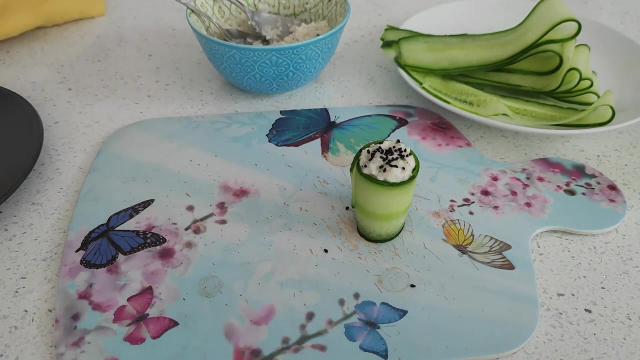 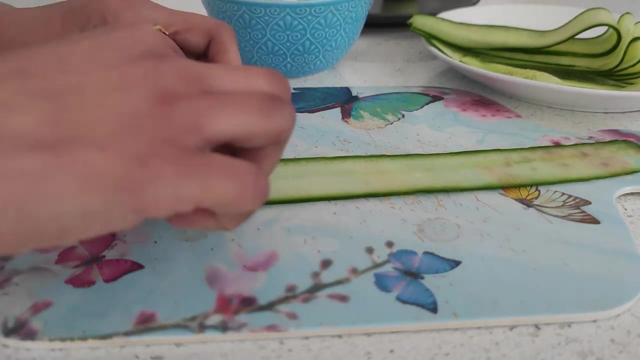 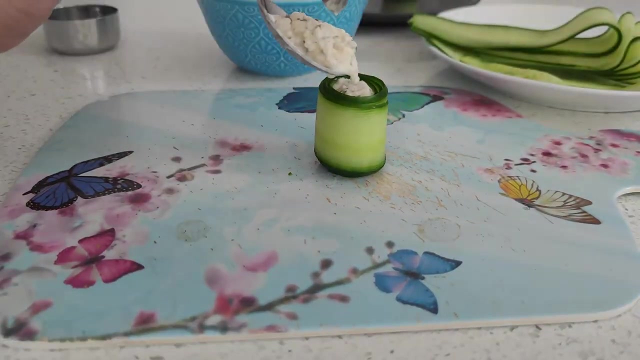 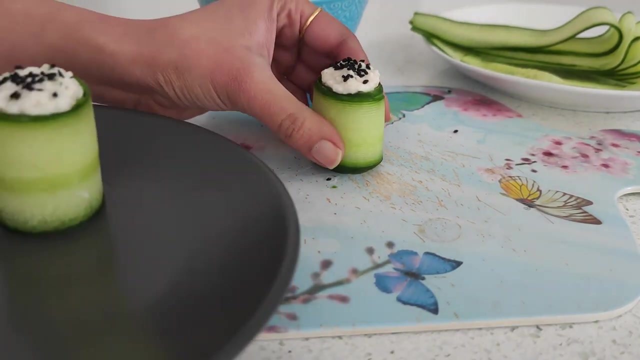 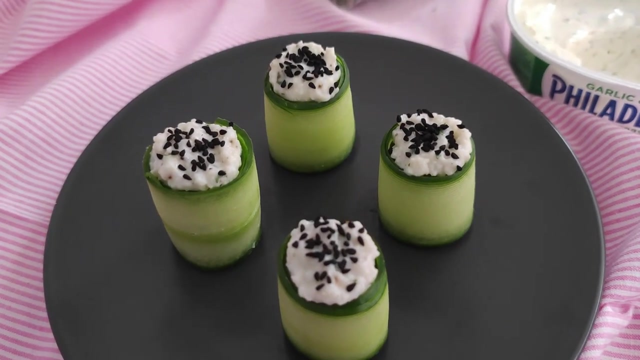 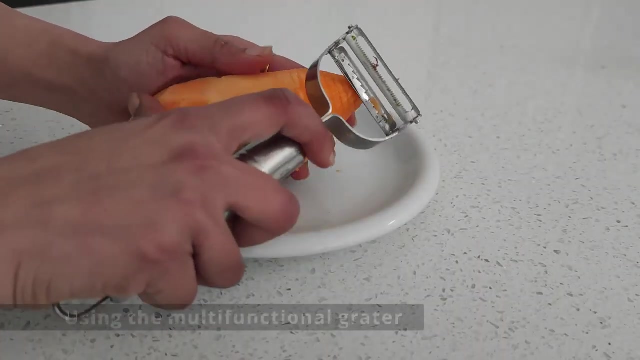 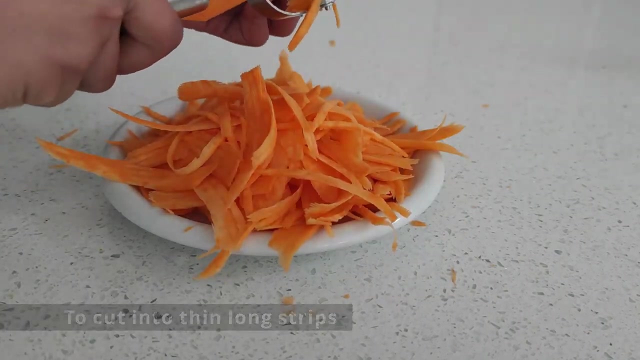 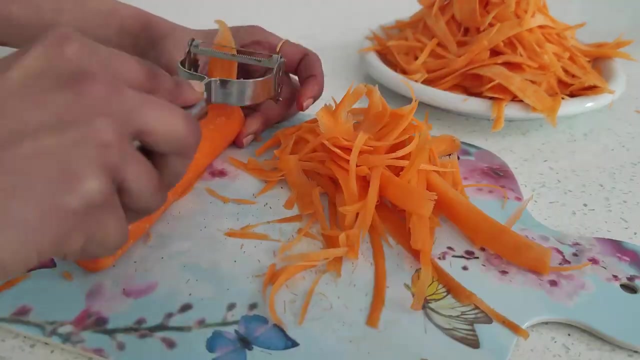